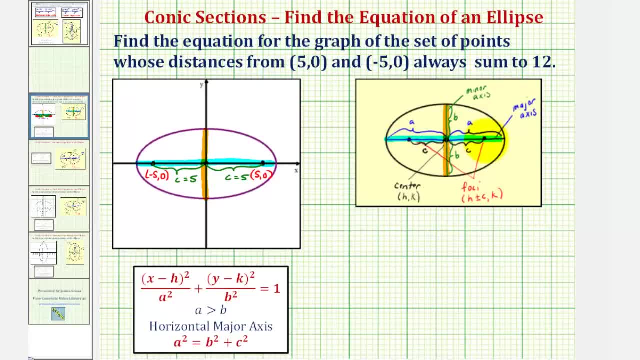 where 2a is the length of the major axis and 2b is the length of the minor axis. Now we're told, our graph is a set of points whose distances from these two points always sums to 12, which means if we select any of these two points, 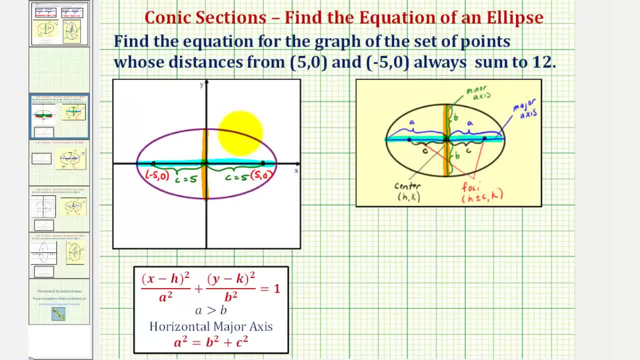 any point on our ellipse. let's just say this point here and find the distance to this focus, and then find the distance to this focus. the sum of the distances must be 12.. So if we call this d sub 1 and d sub 2, for any point on the ellipse, d sub 1 plus d sub 2 equals 12.. 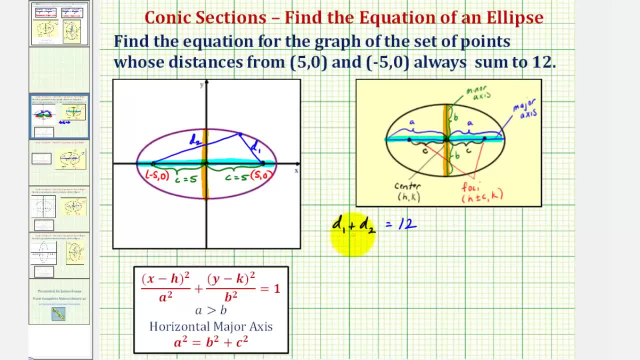 But d sub 1 plus d sub 2 equals 12.. But d sub 1 plus d sub 2 always has the same length as the major axis, which is equal to 2a. So we can say that 2a equals 12.. 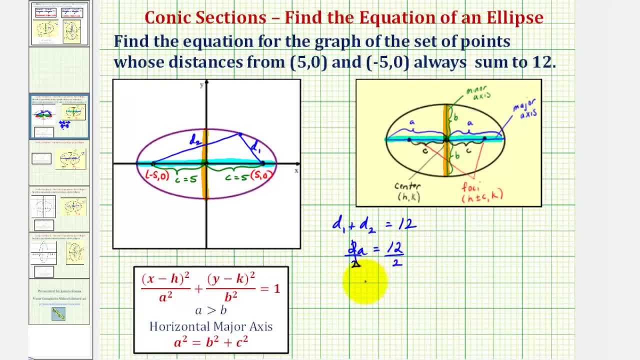 So if we divide both sides by 2, notice that a equals 6.. So we still have to find b. but before we find b, let's try to explain why the sum of the distances would always be 2a. Instead of selecting this point here, let's say we selected the point to be one end point. 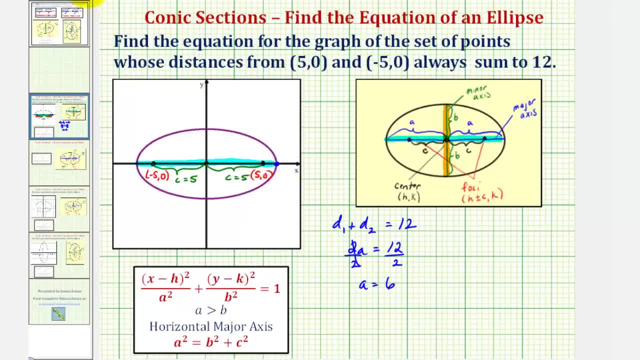 of the major axis, And we know from our notes that this distance here from the center to one end point is equal to a. So notice how the distance from this point to this focus here would be a plus c. So we'd have the quantity a plus c plus the distance to this focus. 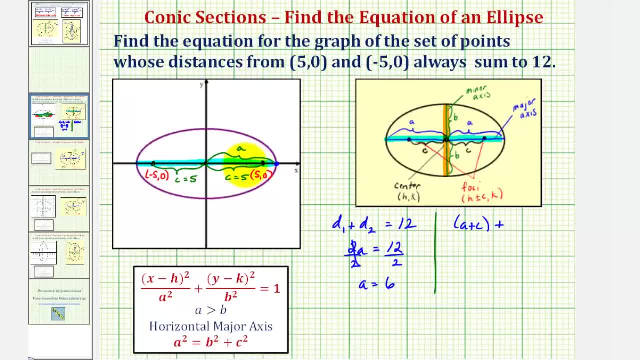 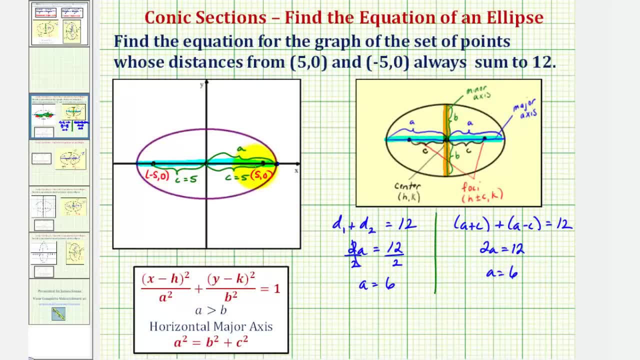 So it is always true, the sum of these two distances is always equal to 2a. Hopefully, this helps explain why, Now that we know a is 6 and c is 5, we still have to find b to find our equation. To do this, we can use the formula a squared equals 2a.